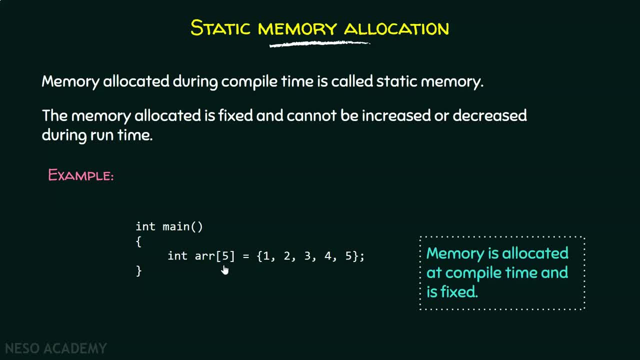 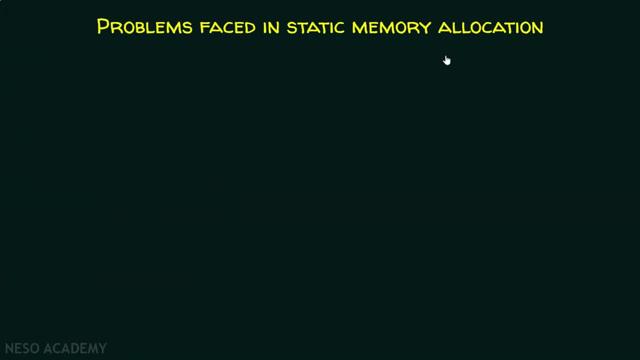 The programmer has fixed this size and we cannot increase this size or decrease this size at runtime. It should be very clear Now. there are certain problems which we faced in static memory allocation If you are allocating memory for an array during compile time. 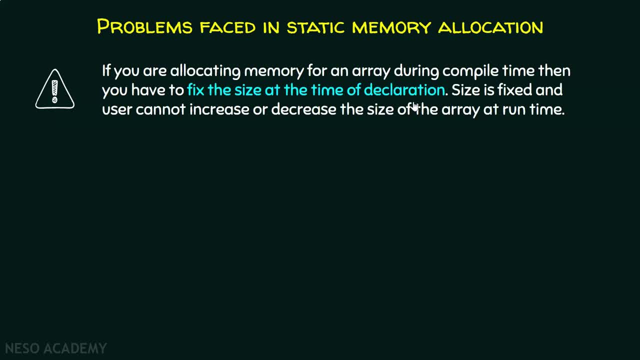 then you have to fix the size at the time of declaration. Obviously there is least flexibility because you have to fix the size at the time of declaration itself. Size is fixed and user cannot increase or decrease the size of the array at runtime. This size is fixed. 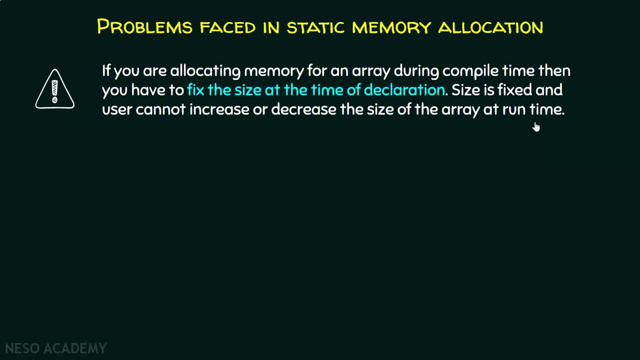 User cannot increase or decrease the size of the array or any object at runtime. If the value stored by the user in the array at runtime is less than the size specified, then there will be wastage of memory. Let me tell you that here I am talking about array. 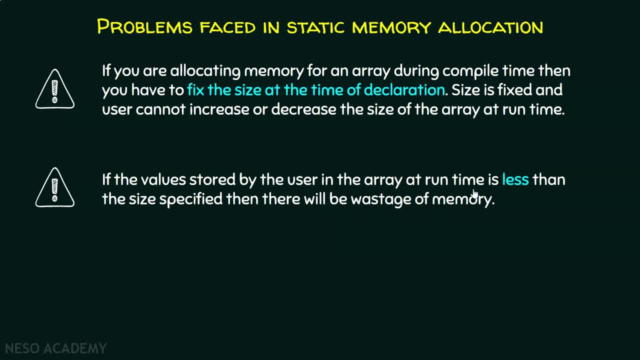 It could be any object, right. So if the value stored by the user in the array at runtime is less than the size specified, if the user enters elements less than the size specified, then obviously there will be a wastage of memory. 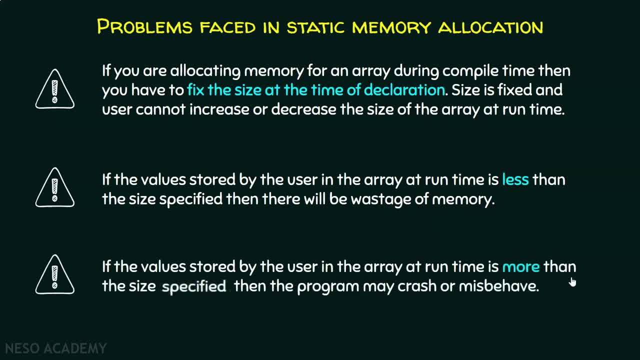 If the value stored by the user in the array at runtime is more than the size specified. if he or she enters more elements in the array, then obviously the program may crash or misbehave. This is also a possibility right Now. here comes a problem. 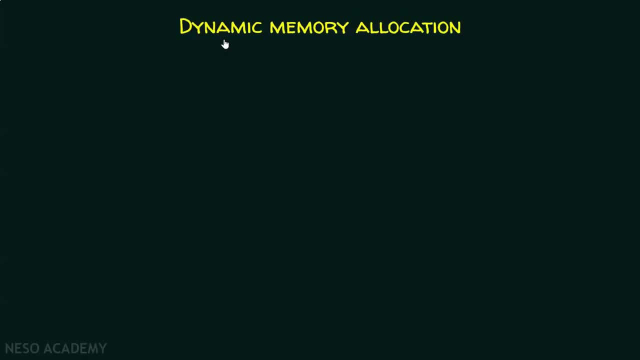 Someone to rescue. The one who can solve the problem is dynamic memory allocation. The process of allocating memory at the time of execution is called dynamic memory allocation. It should be very clear that the process of allocating memory at the time of execution is called dynamic memory allocation. 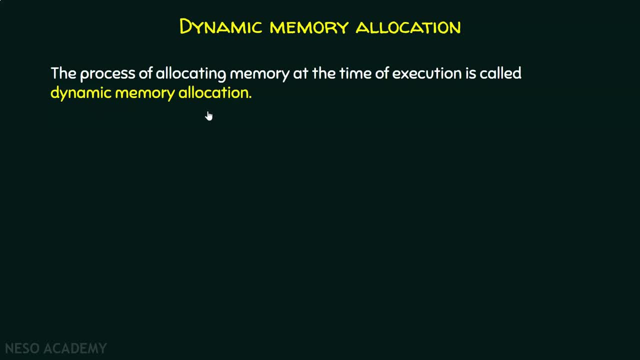 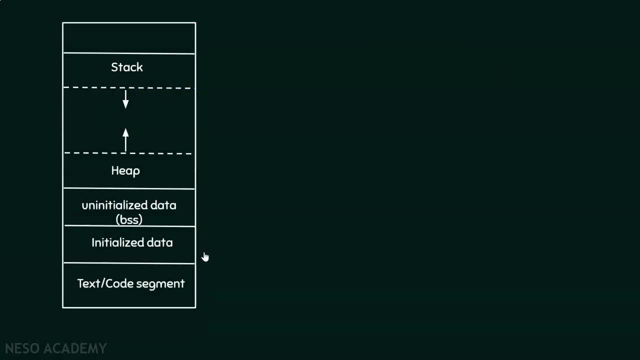 You are allocating memory at runtime, So user has the flexibility He or she can allocate memory according to his or her needs, right? You might have remembered this diagram from C programming lectures. This is nothing but a memory layout of C program. 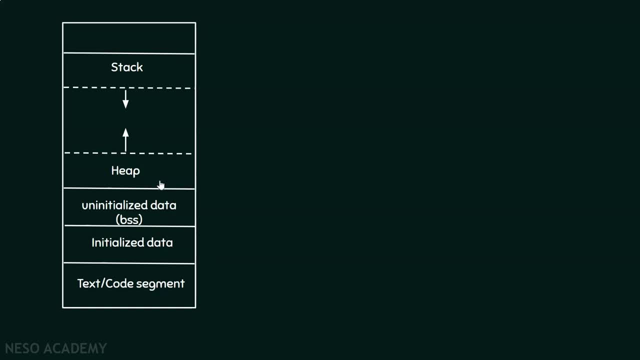 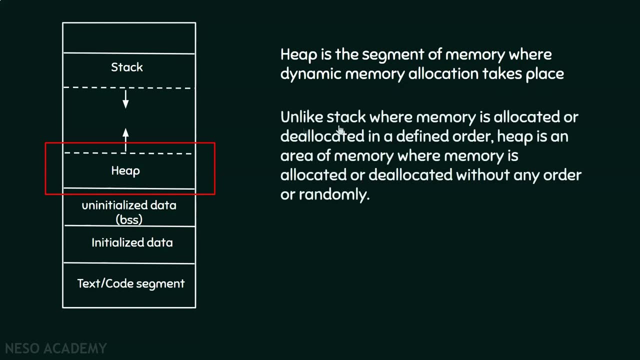 These are the different memory segments. The one which we will talk about here is the heap memory segment. Heap is the segment of memory where dynamic memory allocation takes place. Unlike stack, where memory is allocated or deallocated in a defined order, heap is an area of memory where memory is allocated or deallocated without any order or randomly.